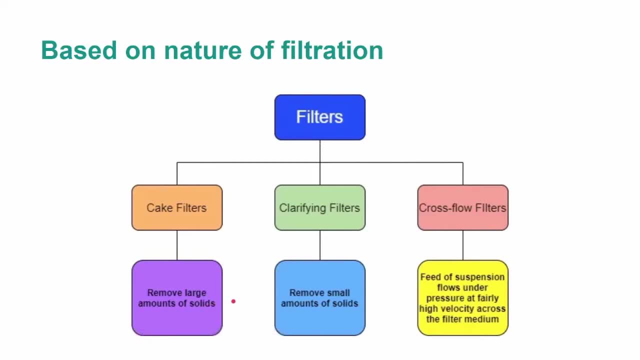 into those details. we next move on to clarifying filters. Clarifying filters are used to remove small amounts of solids or liquid droplets from either liquids or gases. The particles are trapped inside the filter medium or on the surfaces. Moving on to cross flow filters, 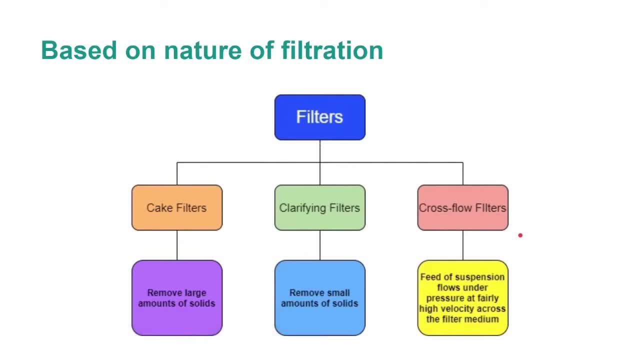 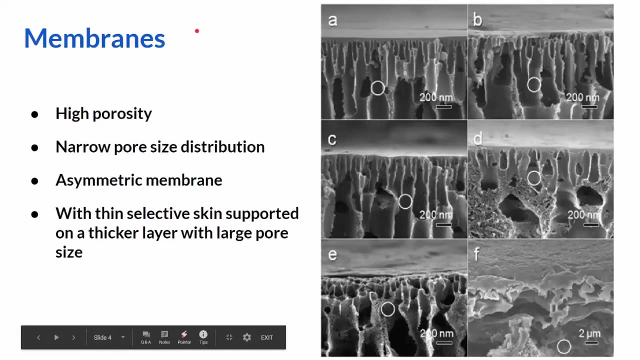 cross flow filters mainly covers those filtration processes where the feed of suspension flows under pressure at fairly high velocity across the filter medium. We come across terms like microfiltration, ultrafiltration, which is our topic, and hyperfiltration. in this type of filtration, As we have seen, ultrafiltration is basically a membrane filtration phenomena. 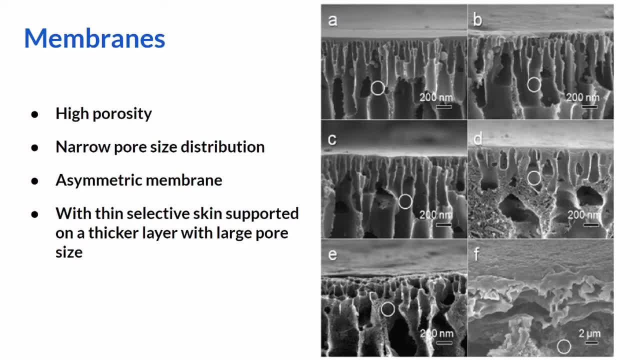 So the nature and quality of membrane would play a pivotal role in it. The membranes should have high porosity, narrow pore size distribution, asymmetric- and generally we tend to prefer asymmetric- membranes with thin selective skin supported on a thicker layer with large pore size. The image on the right is actually a cross sectional view of ultrafiltration membrane. 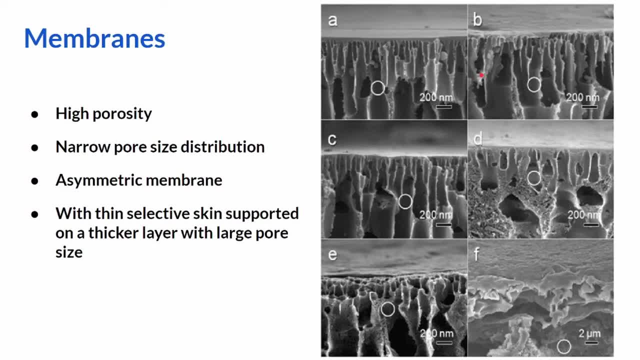 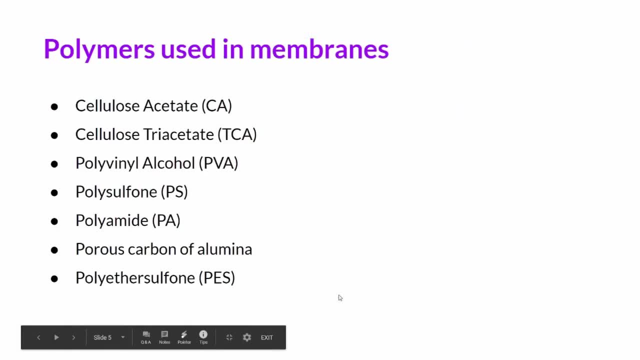 taken from a research paper by Yazoo et al. Here you can see the pores and the partitions of the membrane, Moving on to the polymers that are used in membrane processes nowadays, we do get to see a variety of polymers being used for the same, starting from cellulose acetate cellulose. 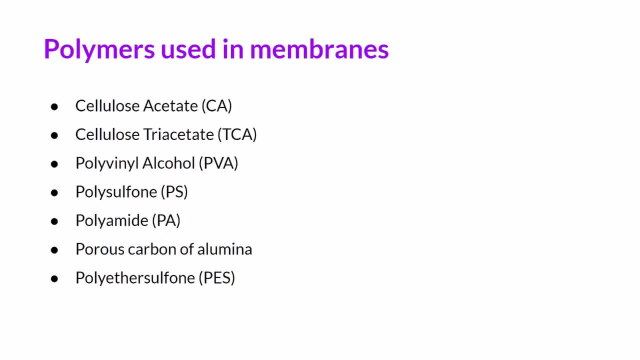 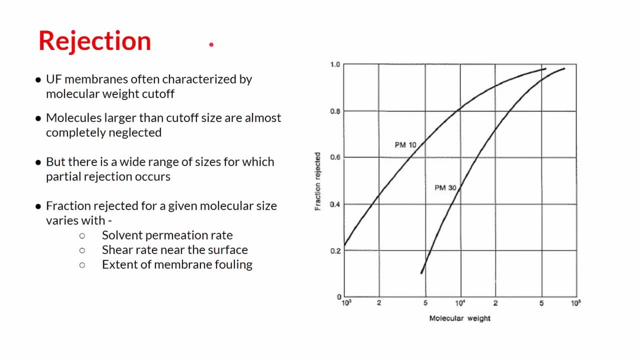 triacetate. polyvinyl alcohol. polysulfone, polyamide, porous carbon of alumina. polyethylsulfone. Rejection is an important phenomena for ultrafiltration membranes, as the ultrafiltration membrane tend to reject particles based on the molecules. 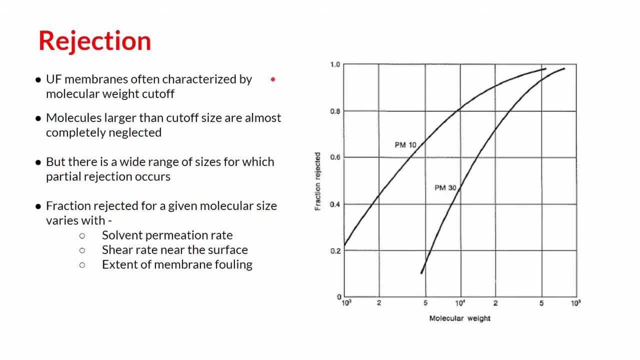 Rejection is an important phenomena for ultrafiltration membranes, as the ultrafiltration membrane tend to reject particles based on the molecules In 5 with 10StT and 30StT for alike. both molecules larger than the cut off size are almost completely. 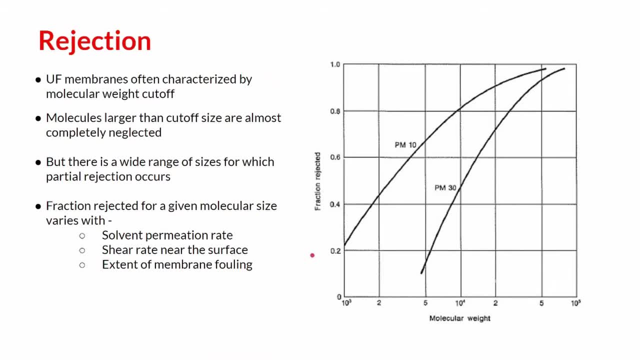 neglected. The graph on the right shows the fraction rejected with molecular weight for 10 and 30 Pm. This has also been taken from a research paper. and word of caution, these data might vary from case to case as fraction rejected for given size varies with solvent permeation rate, shear rate near the surfaces and extent. 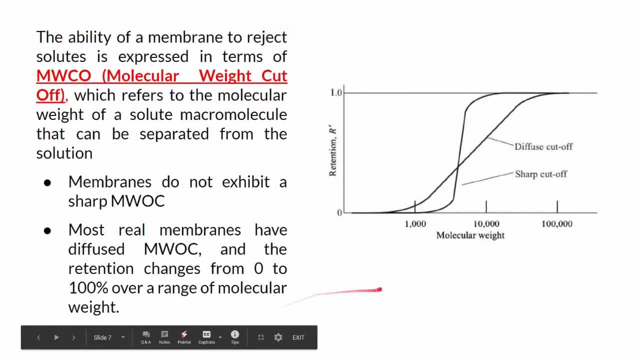 of membrane fouling. As we saw in the previous slide, we can define rejection alternatively as molecular weight cutoff or MWCO, which refers to the molecular weight of a solute macromolecule that can be separated from a solution. In general, membranes don't exhibit a sharp MWCO. 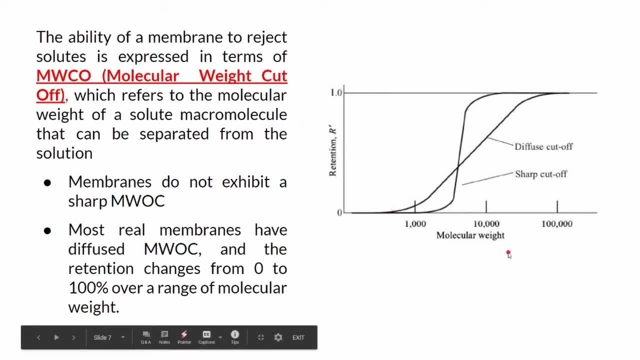 The graph that you see here is actually taken from Datta's textbook. shows a comparison between sharp cutoff membranes and diffuse cutoff membranes. For sharp cutoff membranes, as you can see, the fractional retention almost changes as a step function Within a small molecular range. the retention value changes from 0 to 1.. 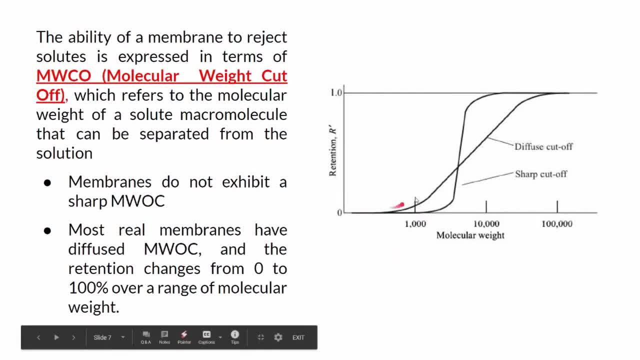 But for diffuse membranes the retention changes gradually over a wider range of molecular weight, as can be seen. So we generally expect most membranes with wide pore size to be technically cutoff Correct to follow a phenomena that is more like diffuse membranes rather than sharp cutoff. 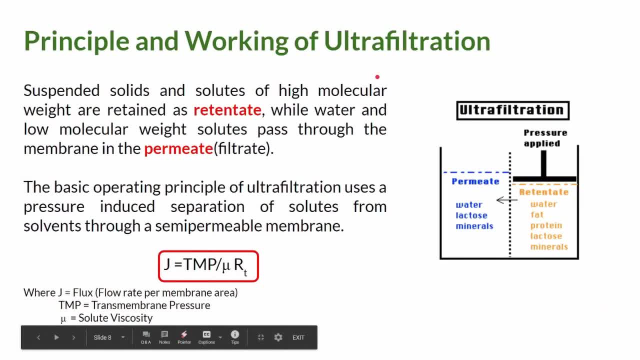 membranes. Before moving on to the crux of ultrafiltration and the formulas, first let's see the principles and working of ultrafiltration. The basic operation of ultrafiltration uses the principle of a pressure induced separation of solutes from a solvent through a semipermeable membrane. 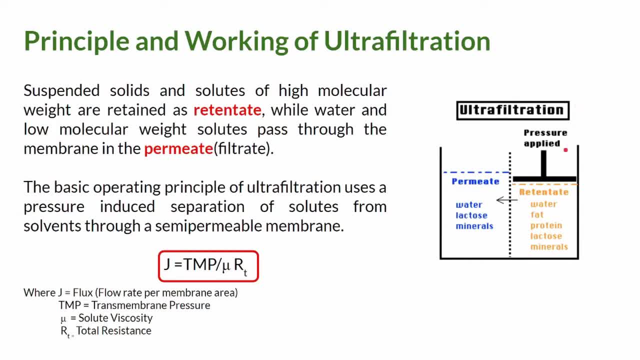 So, as you can see in the diagram, we apply some pressure And the suspended solids and solutes of high molecular weight are retained And water and the low molecular weight solvents pass through this membrane. The solid that is retained by the membrane is termed as retentate, and that that passes 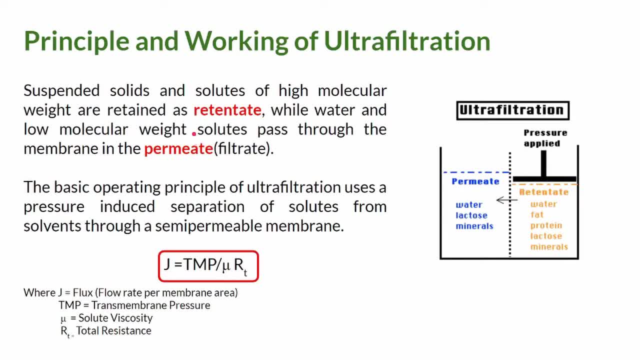 through the membrane is termed as permeate. The relationship between the applied pressure on the solution to be separated and the flux through the membrane is most commonly described by Darcy's equation. As you can see here, Darcy's equation is numerically stable. 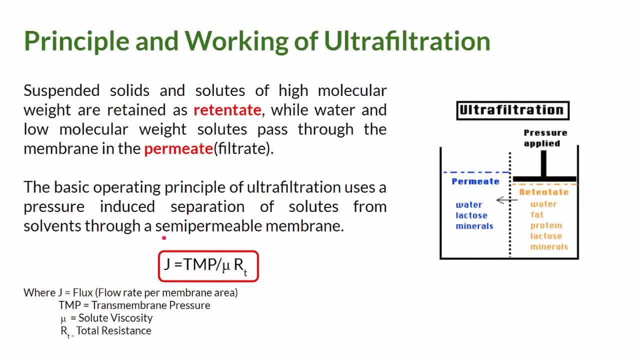 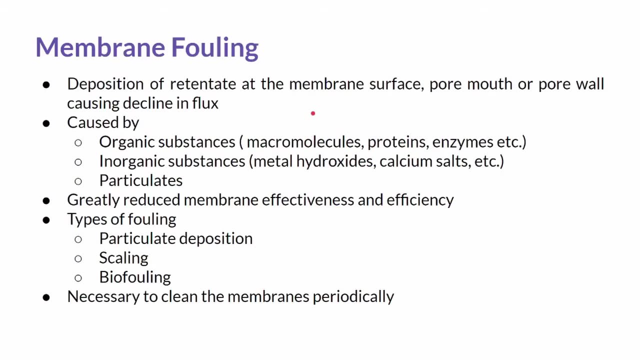 So we can see that Darcy states that J, which is basically the flux, is equal to the transmembrane pressure divided by the viscosity and the total resistance. We will look into details of the total resistance in the next slide. So the total resistance that I was talking about in the previous slide would actually 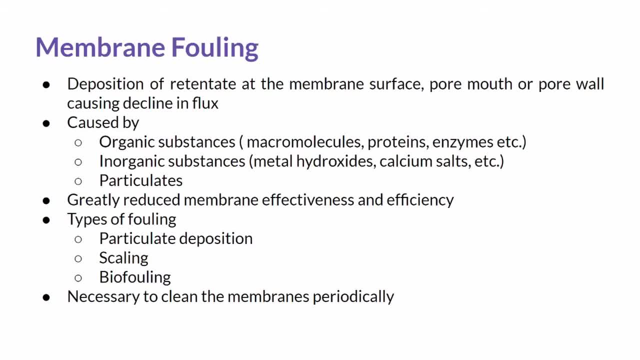 be the sum of the membrane resistance- which is quite obvious to you guys- and the fouling resistance. Talking about fouling resistance would be where We need to talk about the phenomena of membrane fouling. Membrane fouling is actually defined as a deposition of retained particles, colloids. 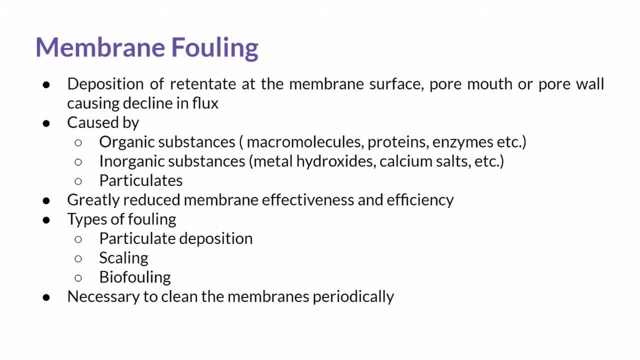 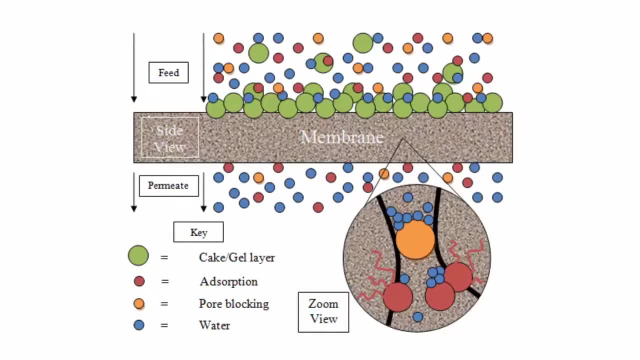 macromolecules, salts, etc. at the membrane surface or on the pore mouth or on the pore wall, causing a steep decline in the input flux. The diagram that you show here, that you see here, is actually the cross sectional view of a membrane. This 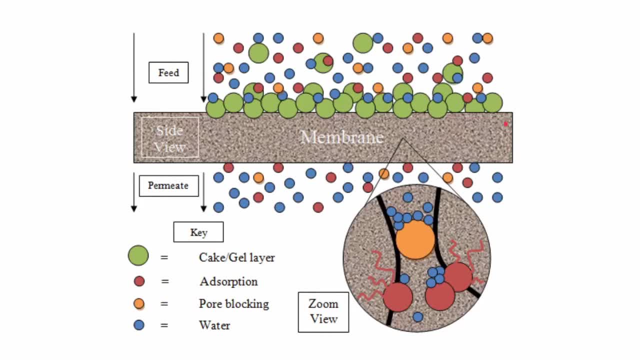 Is The membrane resistance. But besides that we also see a deposition of cake layer. So the incoming water molecules, besides facing the membrane resistance, would also have to face the resistance that is offered by the cake, which we also term as the fouling resistance. 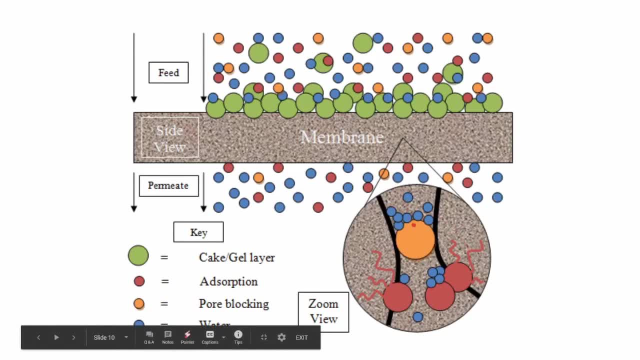 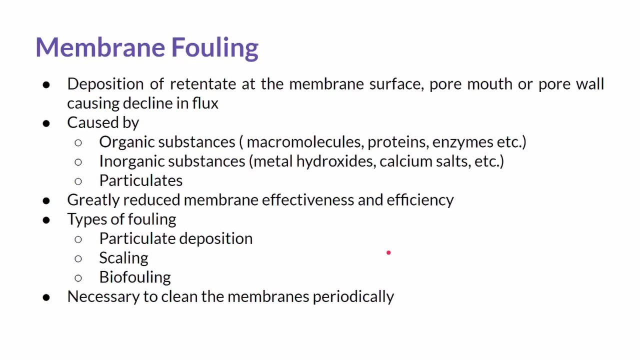 In this zoomed picture you see how the pores are blocked or even sometimes, due to surface configurations, the molecules get adsorbed into the pores, So the pores are blocked And can absorb into the pores, Thus causing resistance to the flow. Fouling can be caused by broadly three kinds of substances. 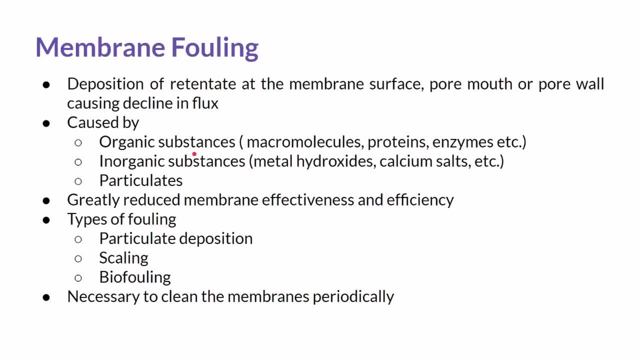 They are Namely organic substances, Which includes macromolecules and biological substances like proteins, enzymes, etc. Or inorganic substances, like metal hydroxides or salts, and particulate or the particulate matter that that may be present In the feed. Moving on, 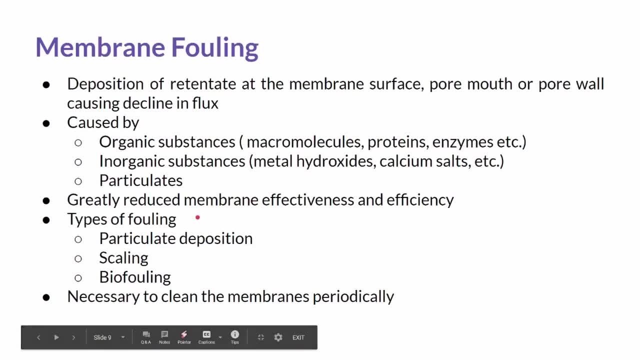 To the to the types of fouling. we mainly have three types of fouling. they are: firstly, particular deposition, which refer to the standard blocking of molecules on the pore walls, pore mouth or the formation of cake layers. then we have scaling, examples of which we have seen our equipment. 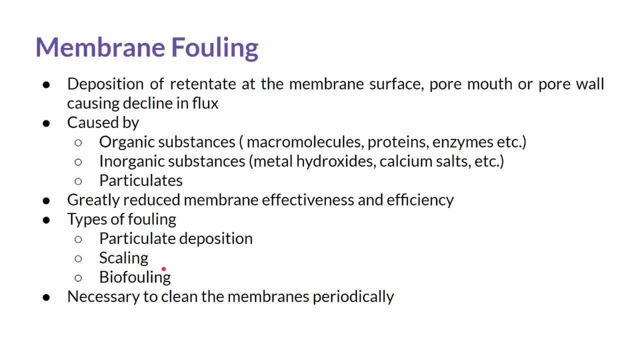 design course. so scaling is basically a result of concentration polarization on the membrane surface, due to which precipitation occurs on the membrane surface. these organic salt deposits block the co pores, causing a decline in the flux. then we have bio fouling, where microorganisms adhere to the membrane surface, forming a gel which is often called as biofilm. these are mostly seen in 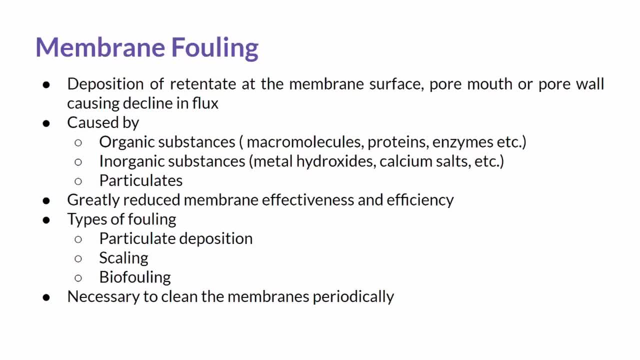 biological equipments or terms related to biology. so, as you might have concluded by now, this membrane fouling is not something that we would desire, and so, time and often, we necessarily need to clean them. with this, we gradually move on to the more mechanical part of the membrane surface, which is called the membrane surface, and this membrane surface is the membrane. 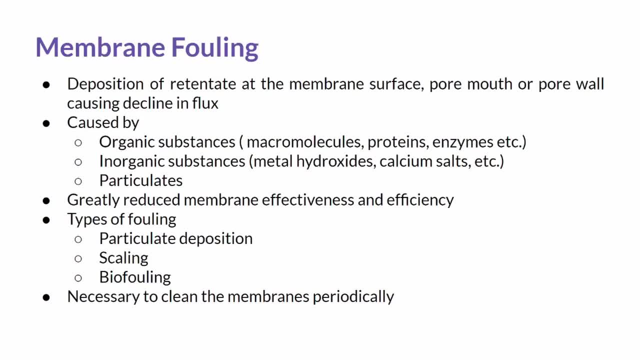 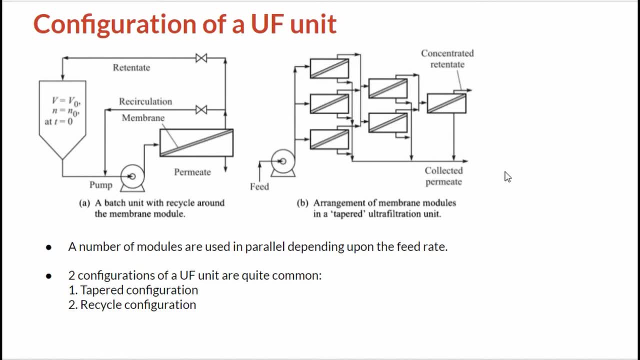 more equation driven part of this topic, through which Lavanya will be taking you on. so now we resume with the configuration of an ultrafiltration unit. in the figure, the two configurations of an ultrafiltration unit, which are quite common, are shown, the second one being the tapered configuration and the A1. 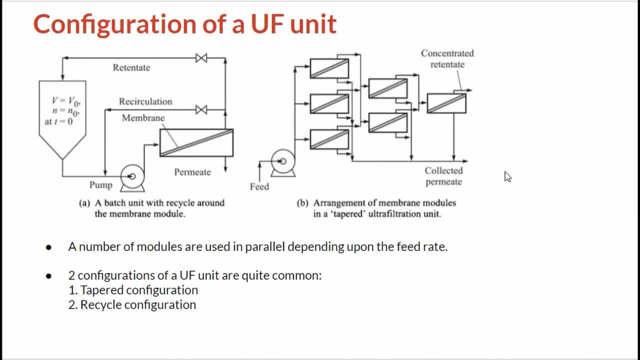 being the recycle configuration. in a recycle configuration, a part of the retentate stream is recycled back to the inlet of the module to achieve a higher concentration of the retentate. the strategy also increases cross flow velocity and thereby reduces membrane fouling. in the other configuration, the 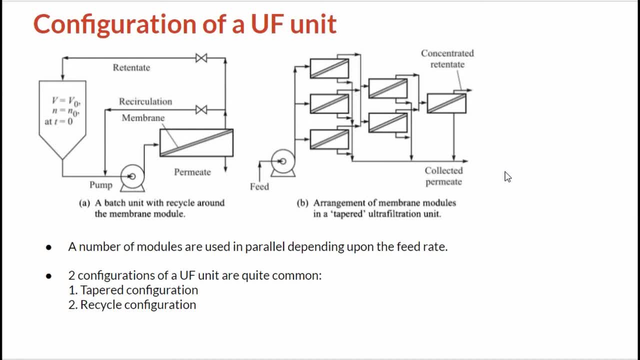 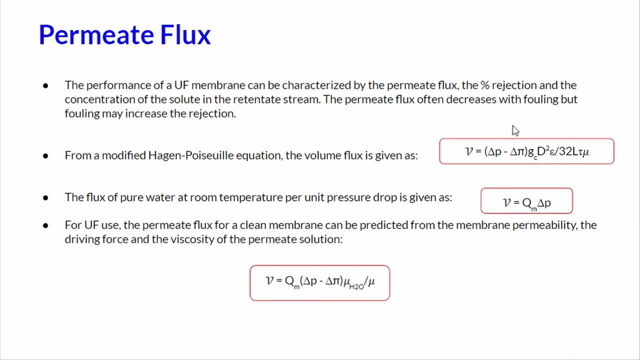 modules are arranged in parallel series pattern. since the retentate volume decreases after the liquid passes through a module, a lesser number of modules is provided in the successive stages. regarding the permeate flux, as we can see, for a clear membrane, the water is assumed to pass through a small pores of the selective layer by laminar flow. 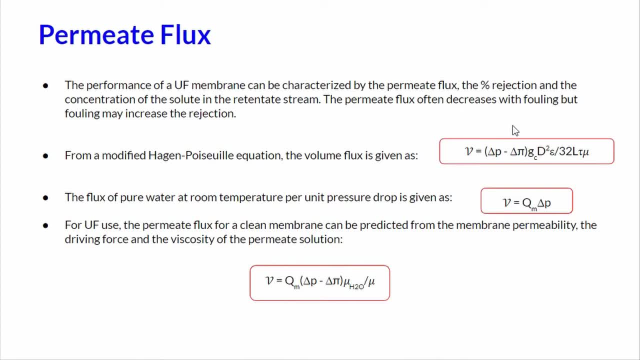 where the driving force is the pressure difference, delta p, minus the difference in osmotic pressures across the membrane, that is delta pi. and so from a Hagen Poiseuille equation, the volume flux is given as the first equation, and for the flux of pure water at room temperature per unit pressure. 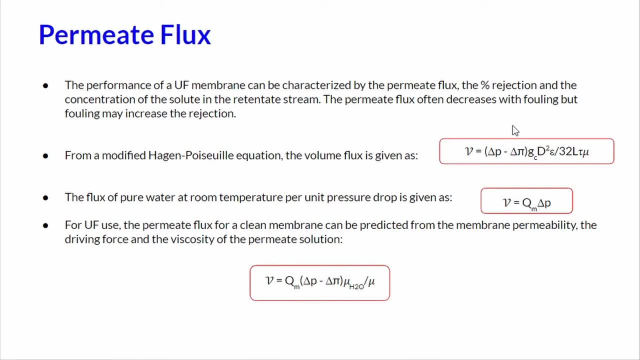 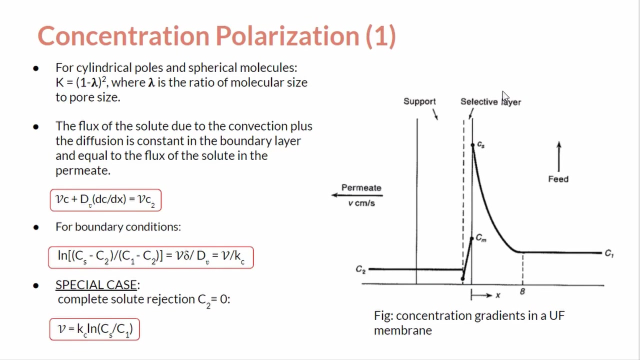 drop is given as the second equation, since it is difficult to get the independent measurements of epsilon D, tau and L for use here. but the corrective can be taken through the membrane permeability QM. now we move on to another important discussion regarding concentration of polarization. does what it pressure difference? delta PI depends on. 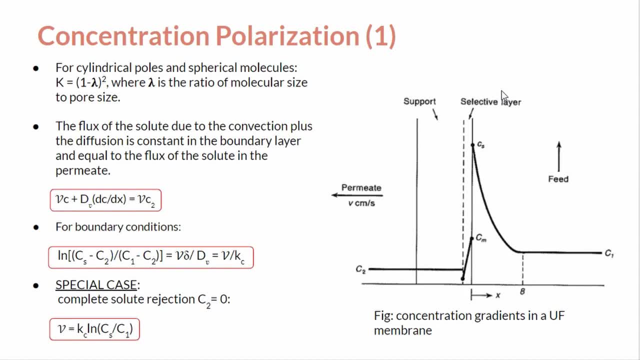 solid concentration at the membrane surface which is much greater than the ball concentration, particularly if the permeate flux is high and the solute diffusivity is slow. the adjoining figure shows the concentration gradients for health. refused rations system with partial rejection of solute: the 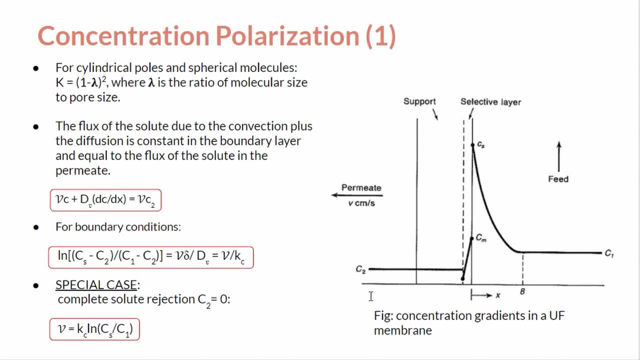 concentration. justice at the pores is newer ten E concentration at the surface Cs. by the factor k, which is the equilibrium partition coefficient For boundary conditions, we obtain the second equation In case when the solute is completely rejected. then our C2 becomes zero and we can use the third equation For lower values of. 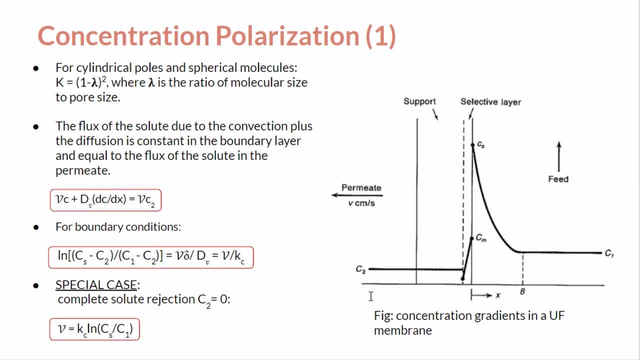 flux Cs can be predicted from the third equation and then using the osmotic pressure data to get delta pi, and delta p can be calculated. If delta p is specified, then a trial and error method may be opted. Through both methods it is concluded that flux should be nearly. 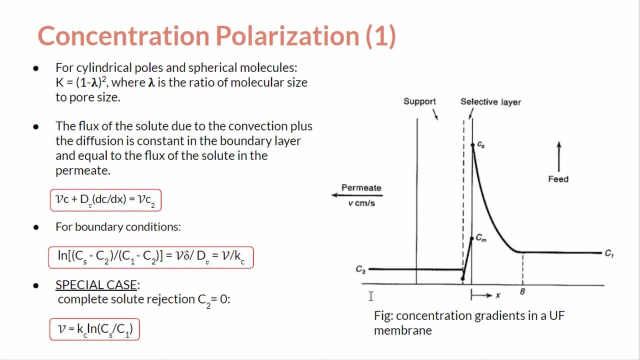 proportional to delta p for lower values of delta p, but the flux changes rapidly with pressure. at moderate pressure ranges The flux eventually changes, reaches a peak independent of delta P, because at that point Cs is equals to Cg, the solubility limit or the concentration at which a gel layer forms. 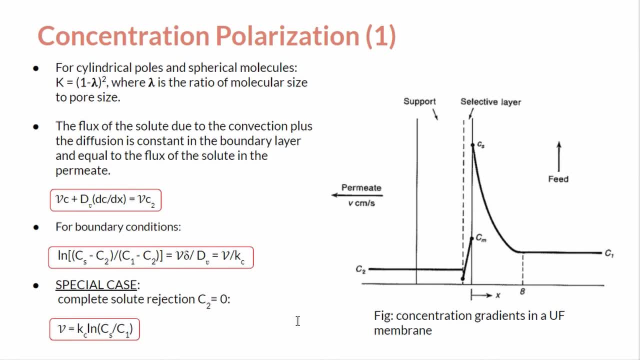 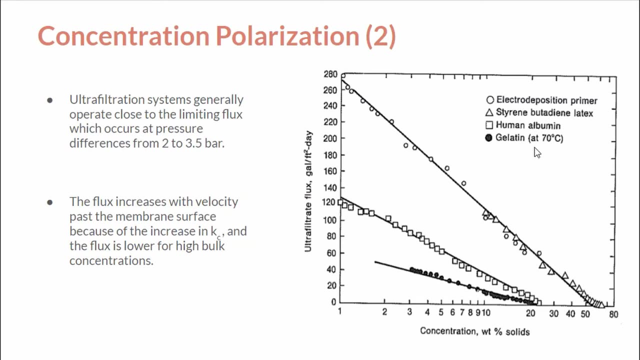 A further sudden increase in delta P gives a temporary increase in permeate flow, but this decreases to a maximum steady state flux as the gel layer becomes thicker and increases hydraulic resistance. Ultra filtration systems generally operate close to the limiting flux, which occurs at pressure differences from 2 bar to 3.5 bar. 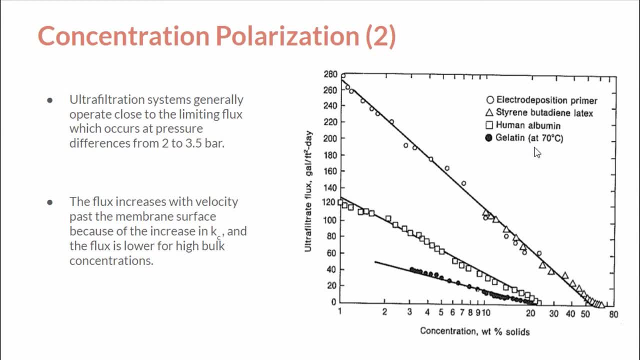 The change in flux width concentration is shown in the figure, and semi-log plots of this type can be extrapolated to zero flux. to determine the value of Cg, The gel concentration ranges from 10% to 50% weight For various proteins and is about 70 weight percent. 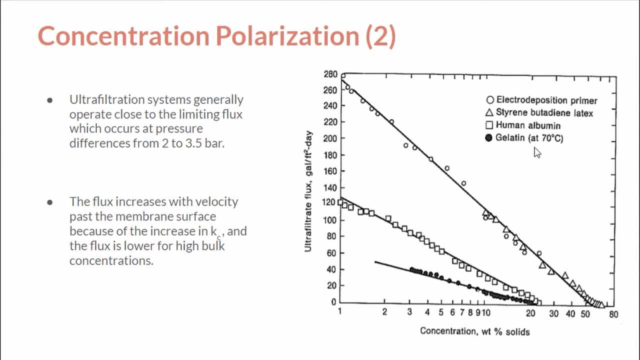 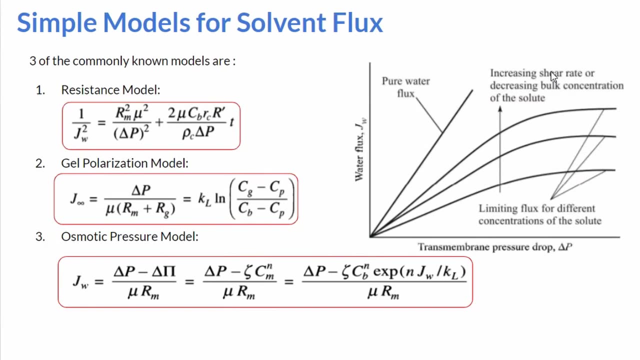 For latex suspensions, the flux increases with velocity past the membrane surface because of the increase in value of Cg, and the flux is lower for high bulk concentrations. Now we move to the topic for simple models for solvent flux. Pure water flux through a membrane linearly increases with applied pressure. 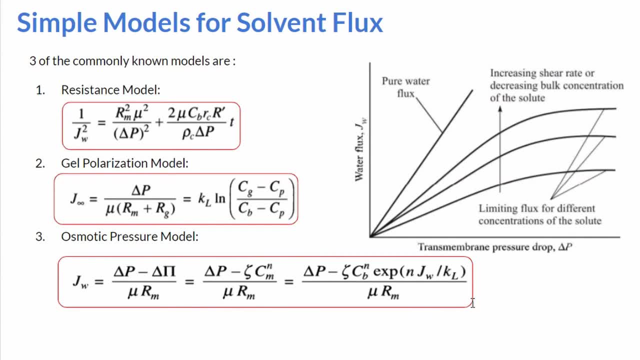 In the case of ultra filtration, however, the increase of flux with pressure drop is slow and the flux levels off to a constant value at high delta P. This constant flux, which is independent of the resistance to flow offered by the membrane, is called the limiting flux. 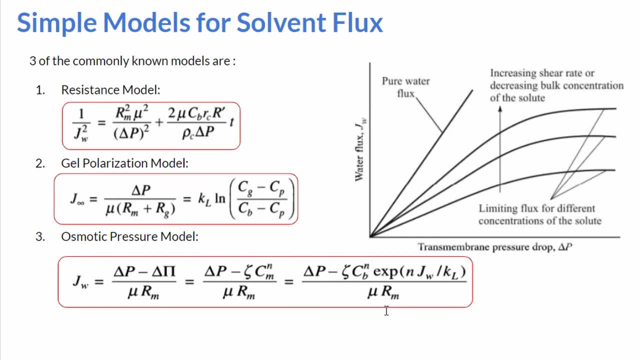 The limiting flux, as shown in the figure, increases with increasing cross flow velocity or decreasing bulk concentration of the solute. Increasing cross flow velocity enhances the mass transfer coefficient and reduces the solute concentration Cm in the vicinity of the membrane. A lower solute concentration in the bulk has a similar effect on the limiting flux. 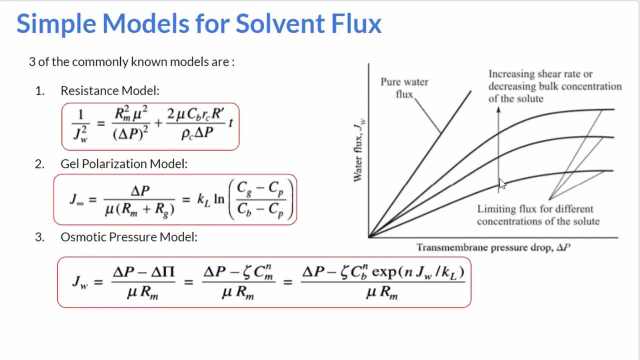 There are three commonly known simple models for solvent flux, the first of which is the resistance model. In this case, a substantial concentration polarization occurs. In the case of high-density flux, the resistance is reduced to a constant value. In the case of high-density flux, the resistance is reduced to a constant value. 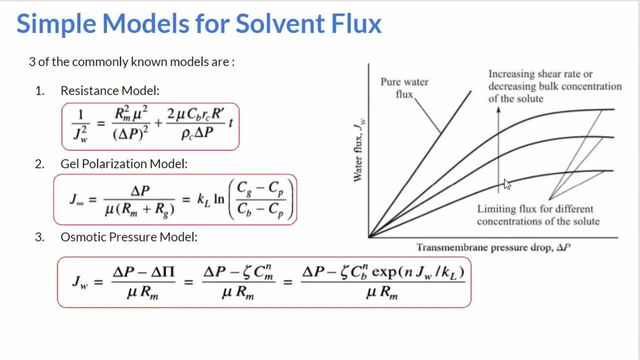 In this case a substantial concentration polarization occurs In ultra filtration. the retained high molecular weight solute may form a thin cake at the membrane surface. The thin cake offers resistance to solvent transport. The equation for the solvent flux Jw can be related to membrane resistance, RM and the 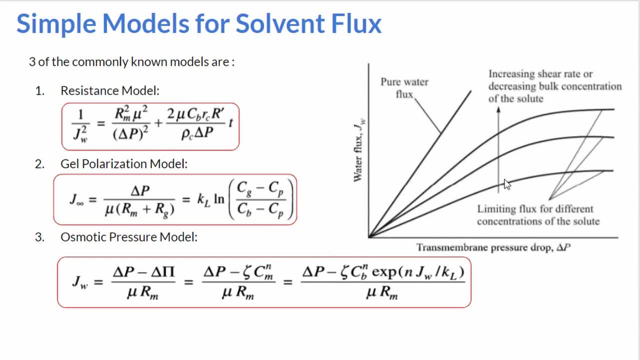 specific cake resistance rc, A plot of 1 over Jw2 versus D for a depth in batch filtration should be linear. The values of RM and rc can be calculated from the slope of the membrane. The thickness of the membrane can be calculated from the thickness of the membrane. 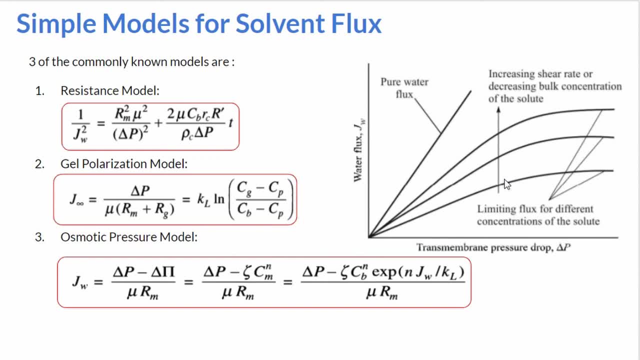 The thickness of the membrane can be calculated from the thickness of the membrane. The thickness of the membrane can be calculated from theWilliam Jw walked the slope into this PrimeUMER ball delta. This can be calculated from the slope of the straight-line plot. 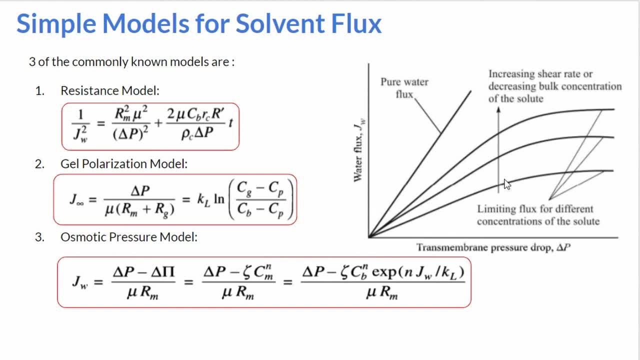 The fit-difference between the source of the tra bidding resistance and the relation of CO release. the followings can be calculated from the slope of the strait-line plot: The resistance for flows through the cake can be calculated using the Kuse-Shen Me Karmann. 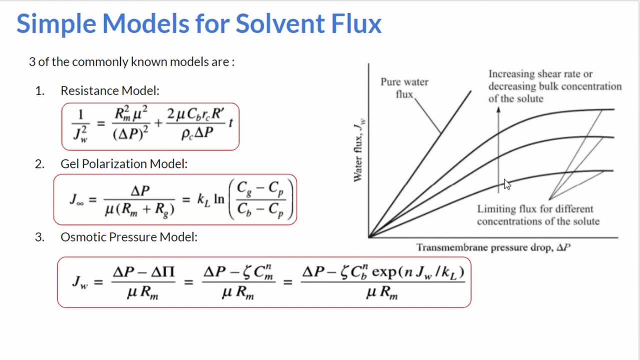 relation. The second one is the gel polarization model. Under the effect of concentration polarization, the solute concentration at the membrane surface may be even an order of magnitude larger than that in the bulk. liquid. Solutes such as polymers or proteins may form a gel if the limiting concentration. 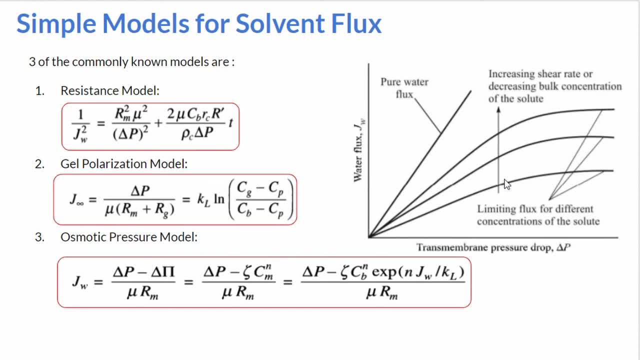 CG is not reached noticeably. If the sanguine surface is wide there may be a lot of venus. concentration cannot be. CG is reached At steady state. a constant thickness of the gel and the limiting flux J infinity are attained When KL is the mass transfer coefficient, the limiting flux is 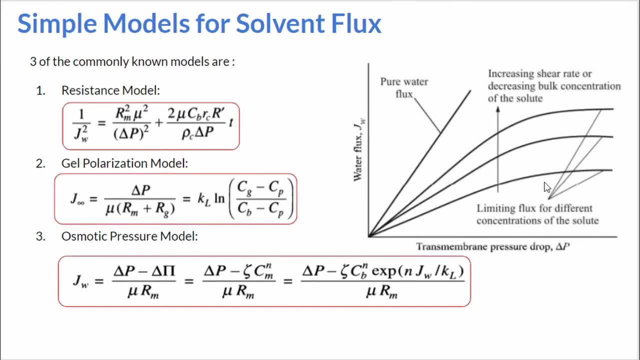 given by the second equation. In the special case that the solute rejection is high, we assume that Cp is very much less than Cb and Cs. Now for the third model, that is, osmotic pressure model. In this case the conclusion is derived from the Van't Hoff equation, and 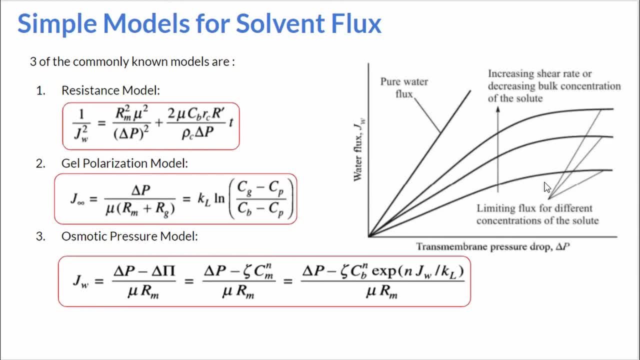 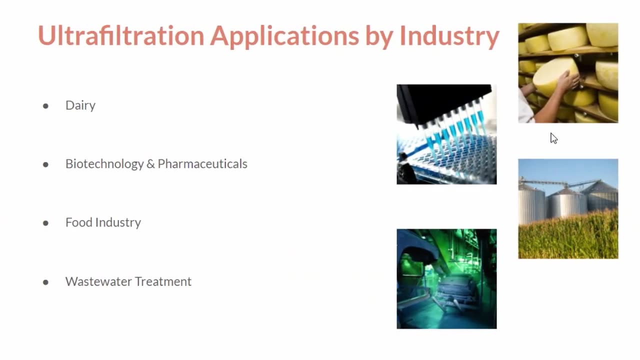 the osmotic pressure of a macromolecule can be described by a power-law dependence on concentration. Using these, we reach the third equation, where the flux is described using the difference of delta B and delta Pi. Now we move on to describe the applications. 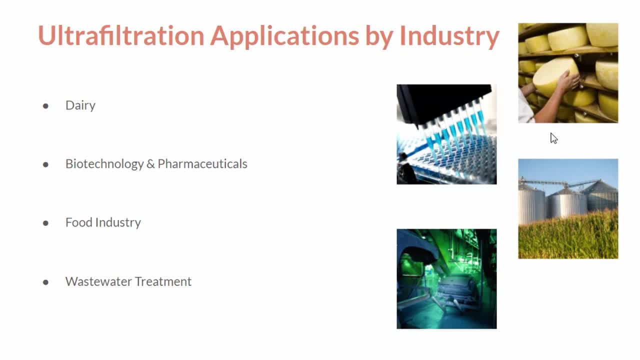 of ultrafiltration, divided by industries. Some of the major applications of ultrafiltration are as follows: The use of ultrafiltration membranes is growing significantly in the concentration and purification of milk proteins across the globe. For biotechnology and pharmaceuticals, ultrafiltration has the 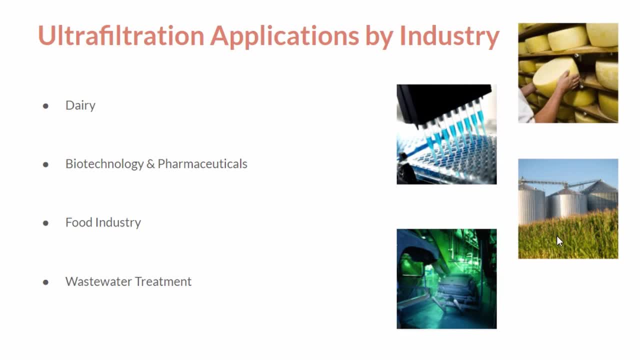 ability to effectively remove pyrogens and endotoxins from solutions, which is critical to the quality control and the production of biopharmaceutical products. In the case of the food industry, ultrafiltration membranes are used for the production and purification. 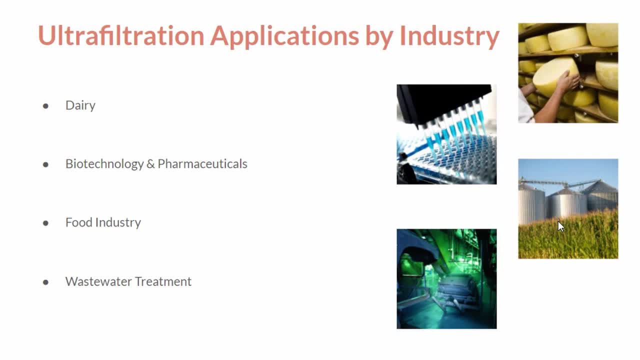 of milk proteins across the globe. In the case of the food industry, ultrafiltration membranes provide optimal flux and retention rates, important for the concentration of gelatin and removal of microorganisms and bacteria, Moving forward with the wastewater treatment industry, in this case with the ability to 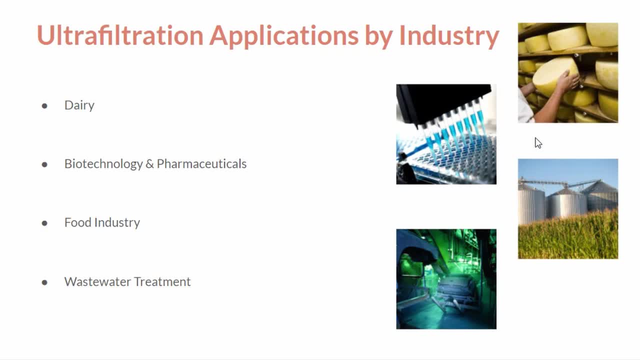 reject particulates, bacteria, proteins and polysaccharides. ultrafiltration can be used in combination with other technologies in the reduction of containment loads and wastewater effluents. And that wraps up the video for us. Thank you for watching. Thank you for watching.